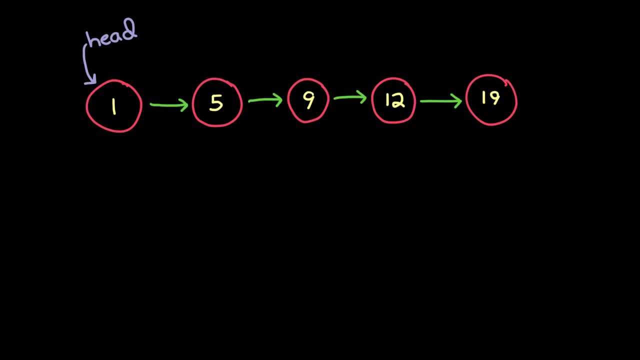 so it's quite a bit slower. So why would anyone use such a data structure? Well, the advantage of linked lists is that they're not always as easy to use. The advantage of a linked list is that insertions and deletions can be very quick, If you just want. 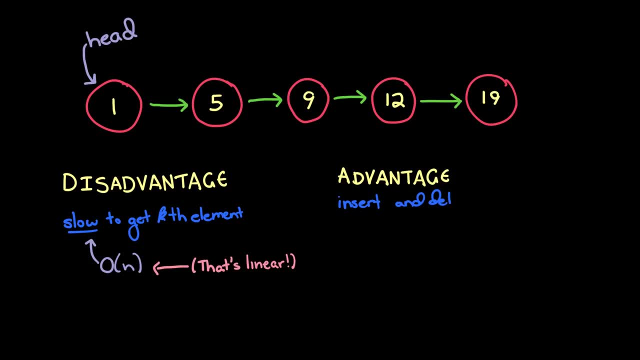 to insert an element right into the beginning of the linked list. that can be done in constant time. If you want to delete an element from the beginning of the linked list, again constant time. So that's very, very fast, Of course, if you want to append an element to the end of the linked list, 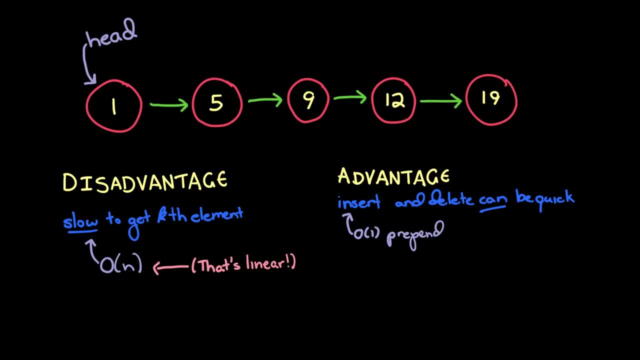 that might require walking all the way through the linked list until you get to the very last element and then inserting the element right into the end of the linked list. Now, there's one other thing we should talk about before we dive into the code, And that is this: 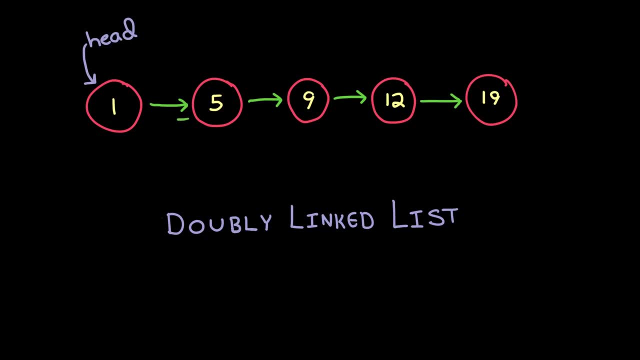 alternate version called a doubly linked list. A doubly linked list is just like a singly linked list, But in addition to each element having a link to the next element, each element also links to the previous element For certain operations. that can be quite handy Now that we've covered. 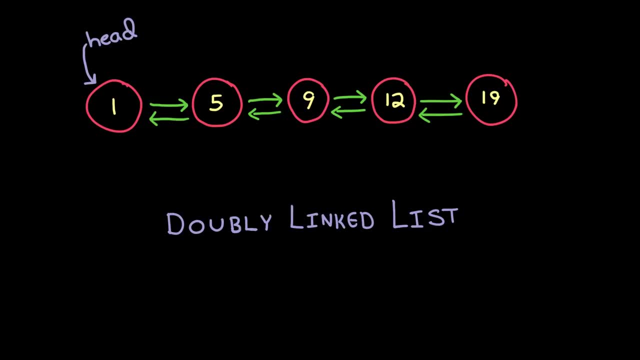 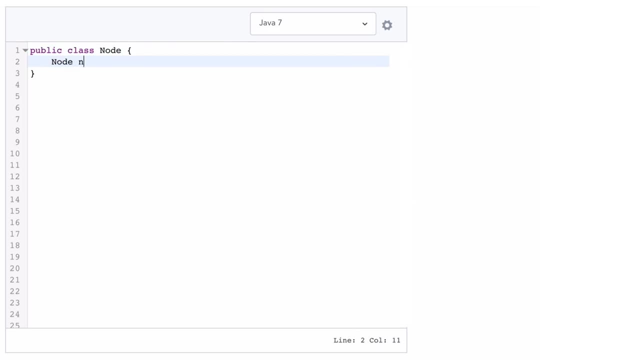 the basics of a linked list. we're going to talk about how to use a doubly linked list. Let's take a look at what the code would look like. Implementing a linked list is reasonably straightforward. We just need a class node that has a next value and a data, And then just to make. 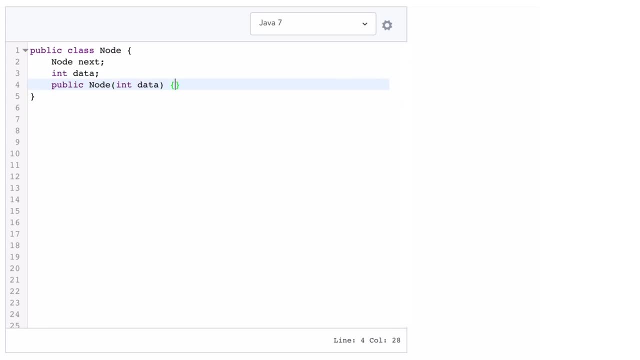 our lives easier. we'll add in a constructor and set that value, Okay. So the first method we'll want to implement is an append method. So let's go ahead and get started with that. Append is going to be a value And then it's going to have some pointer that starts off at the current node. so the 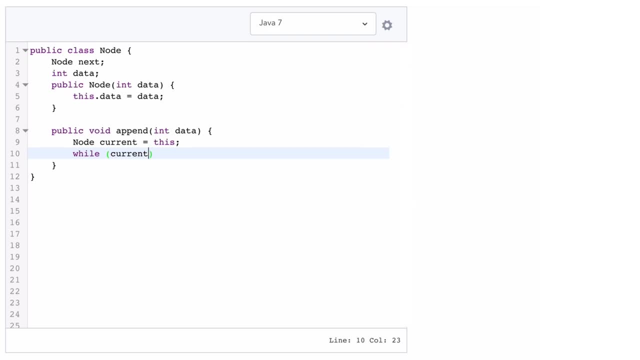 head of the linked list And then it's going to walk through the linked list until we get to the end of the linked list. Well, how do we know that we're not at the end of the linked list? Well, we're not at the end of the linked list as long as there's something after it. So in other words, 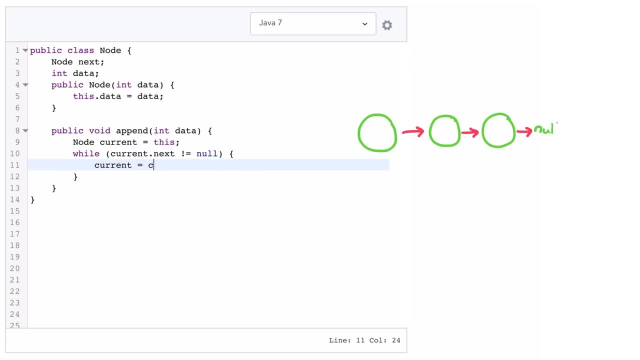 while currentnext does not equal null. keep moving. get to the end of the linked list. Then we get down to the end of the linked list. create this new node. If we prepend an element, we're going to actually change what the head node is. Now this makes a little bit of an issue because 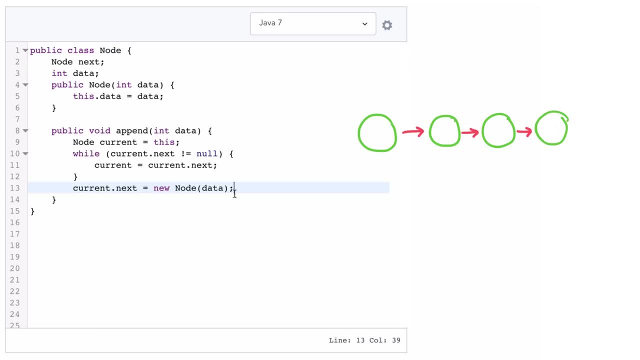 we could have multiple places in our code base that all link to the same head, But if we change the head in one place, how does everybody else know that our head value changed? So the workaround for this is, rather than giving everybody an access to the head pointer directly, we're going to 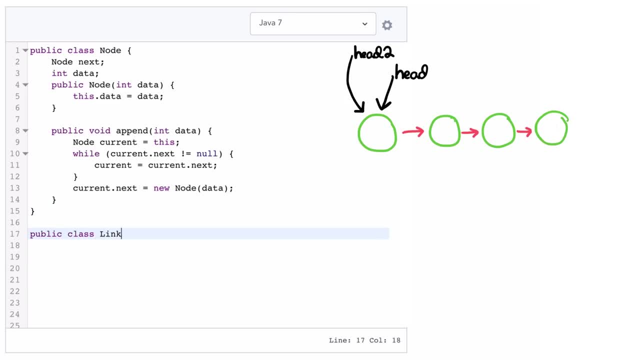 define a class linked list. that's basically going to wrap our head. And then this append method can go where it probably should have from the beginning, which is in this linked list class. And let's just update this because the current node should actually point to the head And what's nice. 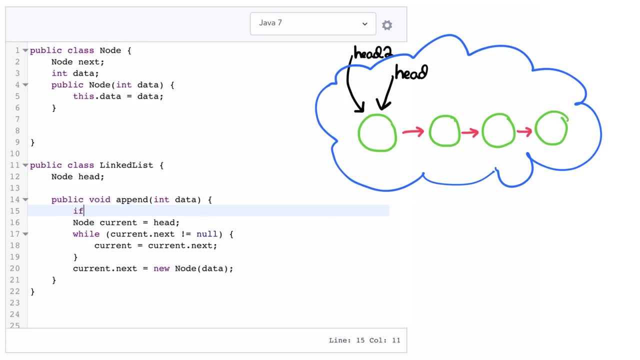 here is that we can also add in the case if the head is null. So we can say: if the head is null, then actually we just want to create the head. So if head is null, head equals new node data, And then we can. 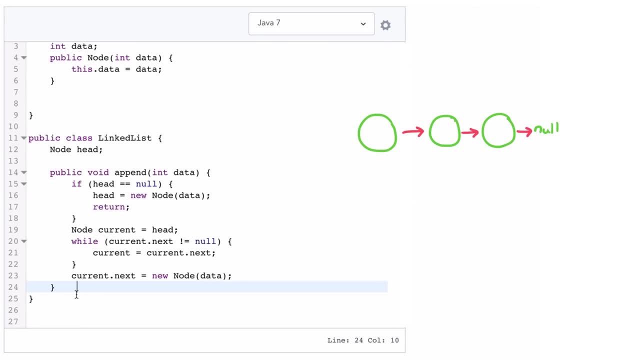 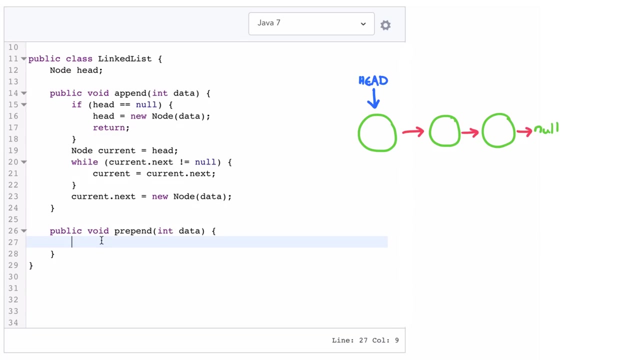 just return because now we're done with that. All right, Prepending is relatively easy. now We just need to, so it's going to be void again. prepend taken data. Now the way this method will work is that we're going to create actually a new head, And what we're going to do is we're going to go. 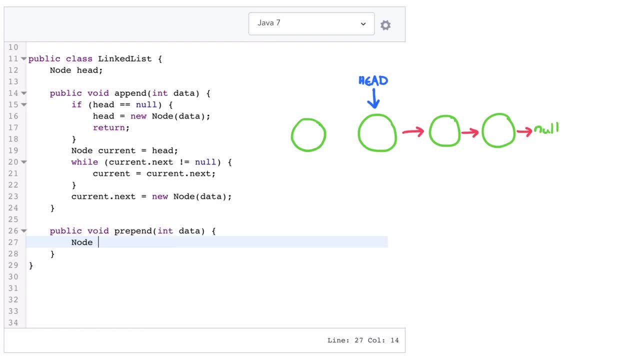 actually a new head value. so node new head equals new node data, then new heads. next value is going to link over to the old head and then we need to change the head pointer. for a final operation, let's implement a method delete- that deletes the first node that has a particular value. so first we'll just declare our. 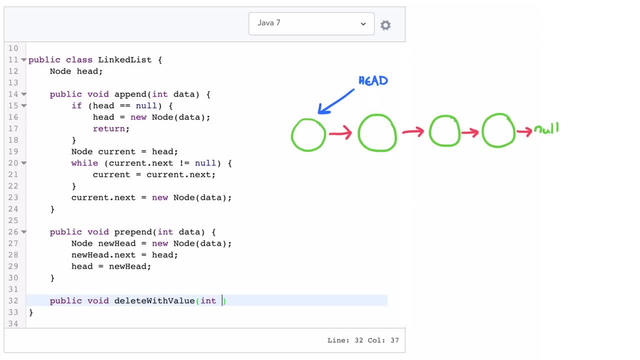 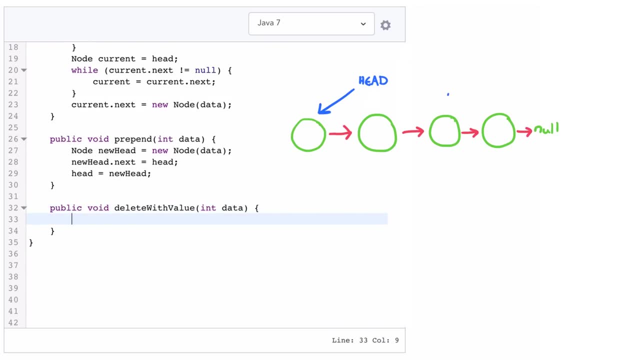 method void: delete with value that takes in a data piece of data. okay, now if head is null, we know we just want to return immediately. there's nothing we can do there. now, what delete with value is going to do, is it can, is it's going to walk through the linked list and it's going to stop one before the element. we. 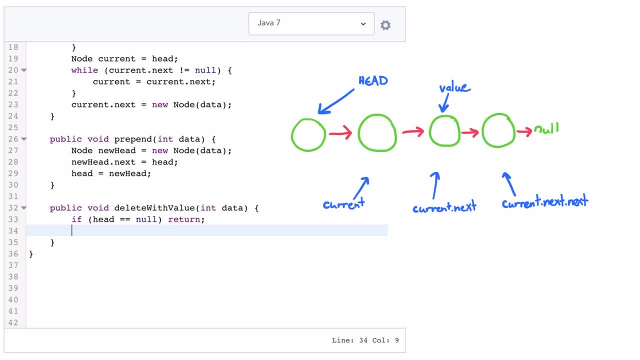 want to delete, and then it's going to say: oh, the very next element you want to delete, so I'm going to delete this one. and I'm going to delete this one actually just update my pointers to work around it. so my next pointer is going to be that: deleted values, next pointer. so let's see how this works. so 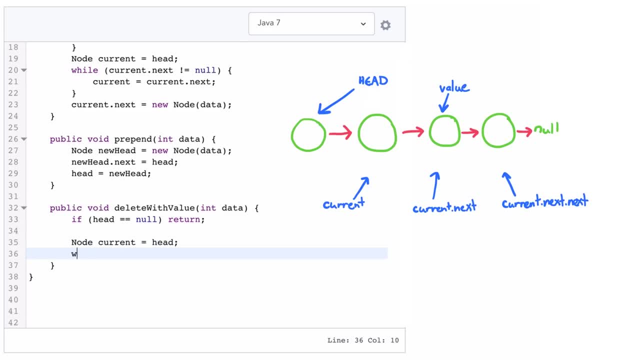 first we'll have this little current method that walks through the linked list, and then we're gonna walk through as long as we're not at the last element, so we don't want to run off the edge of the linked list. okay now, if current dot, next dot, data equals. 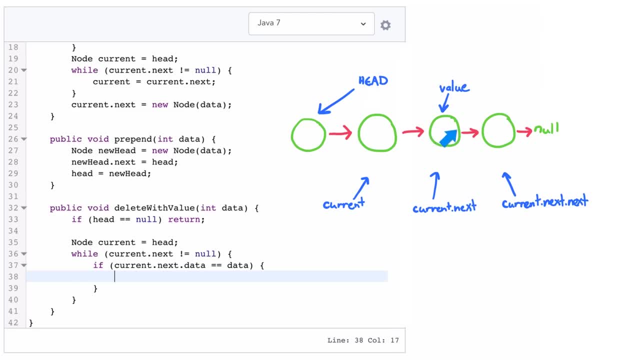 the data we're trying to delete. so in other words, if the next value is the one you want to delete, then cut out that last, that next value, so then current dot next equals current dot next to next, and then we return. so what this is doing is 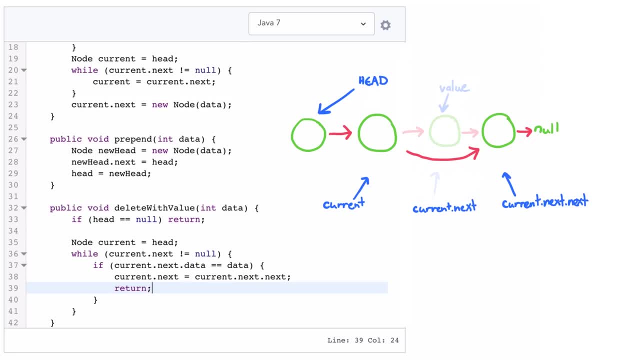 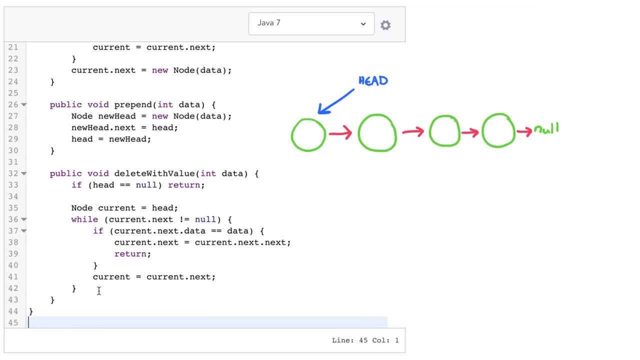 saying: okay, if the next value you want to delete, don't go to that element and just walk around it. set my next pointer to be my next pointers, next pointer, so walk around it, and then in other cases we just move on to the next element. now there's one case we want to be very careful of here, which is what happens if 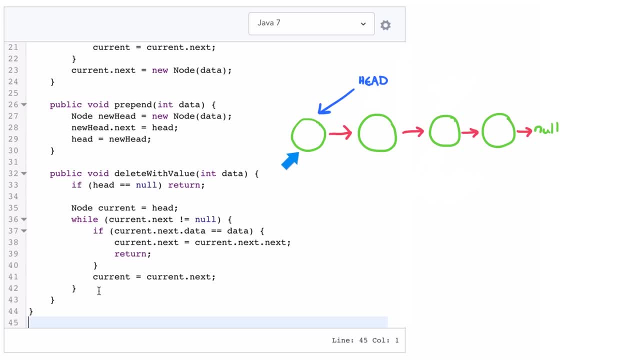 the node we want to delete is actually the head node. this will actually cause a problem- our current scenario- because we need to actually update the head value. so we can just special case that if head dot data is the data we want to delete, then head equals head dot. next, that is just cut me out of the linked list. so now, 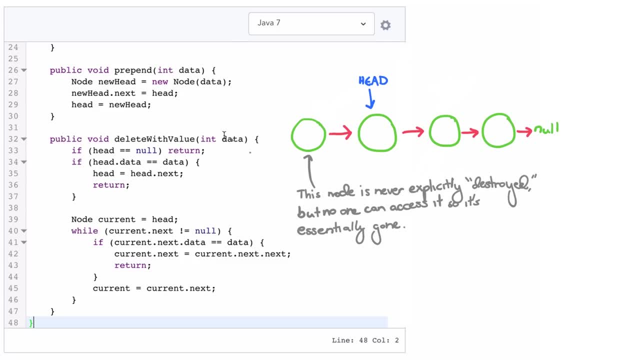 let's take a look at what our method does. so first it takes in this data and then says, okay, if head is null return, there's nothing we can do. if we need to delete the head, then just go and delete it. set head equal to head. dot next set. 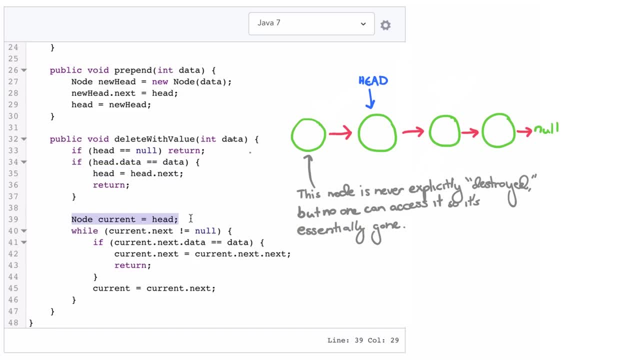 equal to the next value. otherwise walk through the linked list, starting at the head value, then, as long as you walk up until the next value is the one we want to delete, in which case we say, okay, set current dot next, my next pointer, over to the next next value, and then we return, otherwise we continue walking. 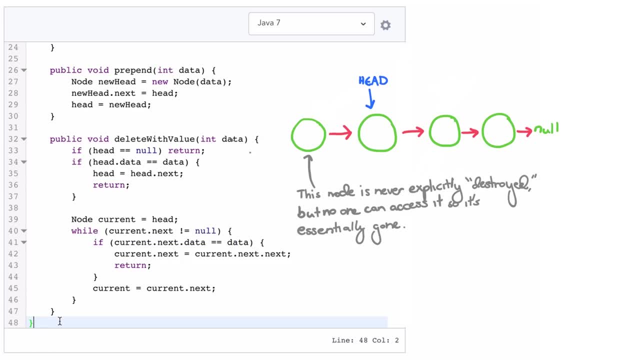 through the linked list. so those are the basic operations for deleting, inserting both appending and prepending into a linked list. now that you've seen the basic operations, why don't you give it a shot on a new linked list problem?